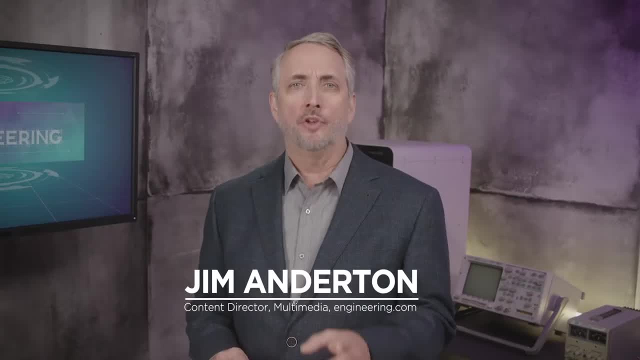 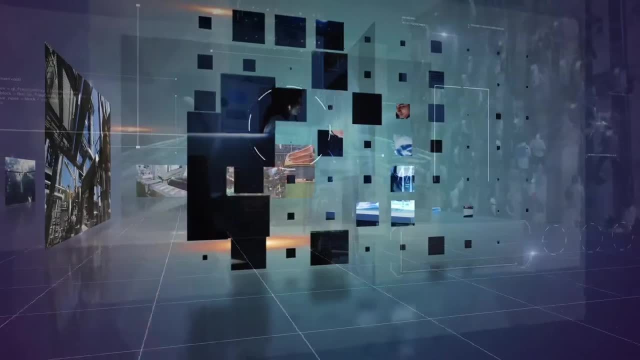 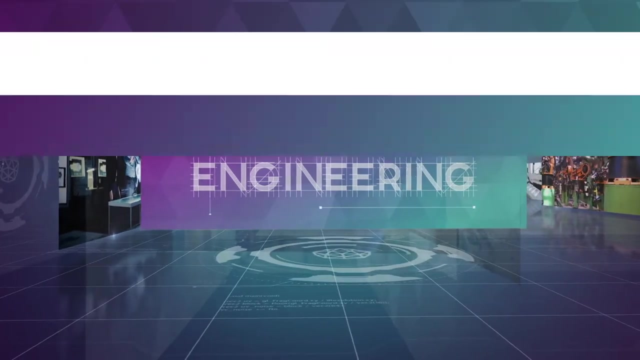 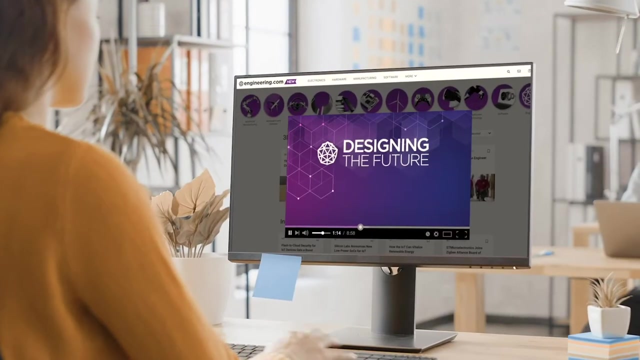 On today's episode we're looking at semi-solid casting and trends in the global automotive die casting market. That's This Week in Engineering. Today's episode is brought to you by Engineeringcom, the world's trusted source for engineering content. Check out this and many other videos for the working engineer on engineeringcom. 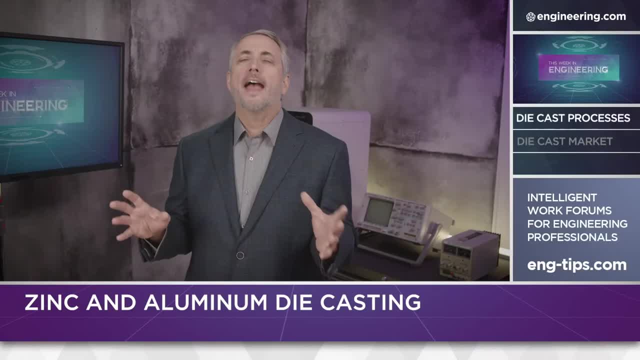 slash TV today. You know die casting has been around a long time for zinc and aluminum bearing alloy small part production. Now it's always been a go-to technology when dimensional accuracy with big volumes were needed. Die casting can accurately produce complex components and high performance. 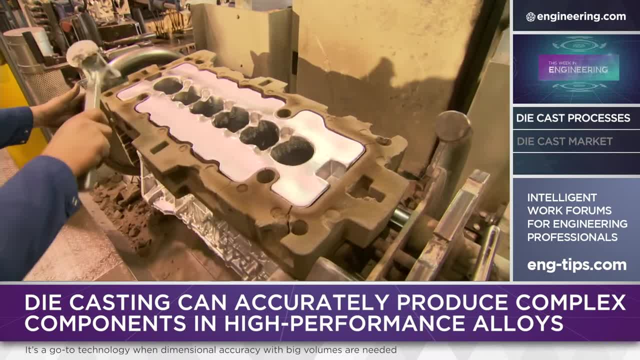 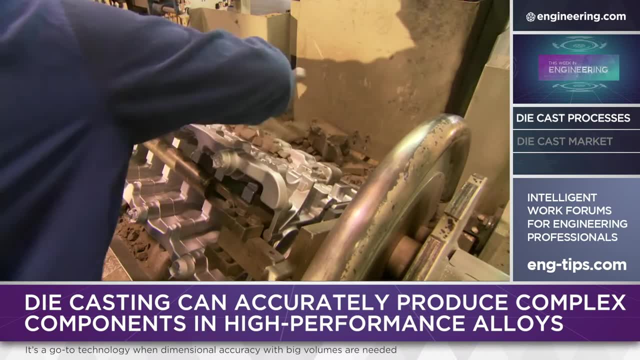 alloys with fine grain structures. but it has some limitations. Flash at the mold, parting lines, knit lines, sink marks, ejector pin marks, shrink and distortion and notably porosity are all dependent on die design, machine parameters and good feedback. 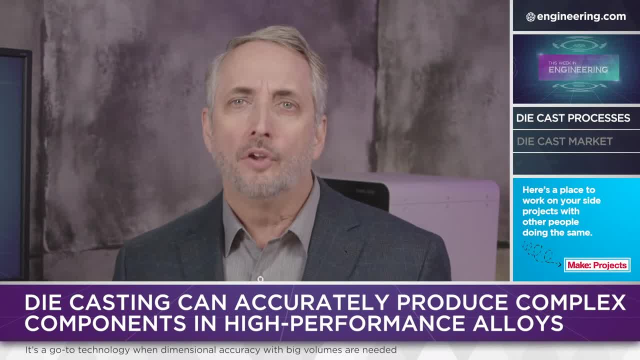 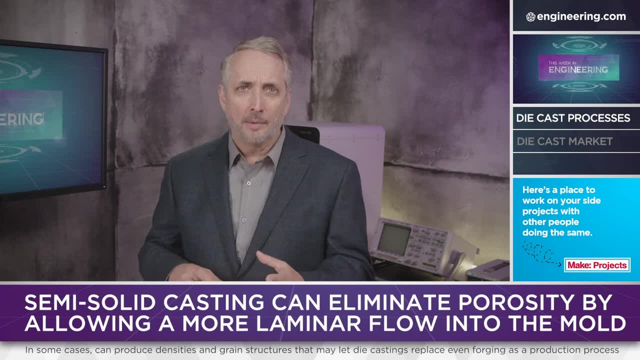 Now gas is entrained in the alloy due to the turbulent flow entering the mold. Well, that can be a serious problem when porosity is an issue. Semi-solid casting, however, can really reduce porosity by allowing a more laminar flow of metal into the mold. 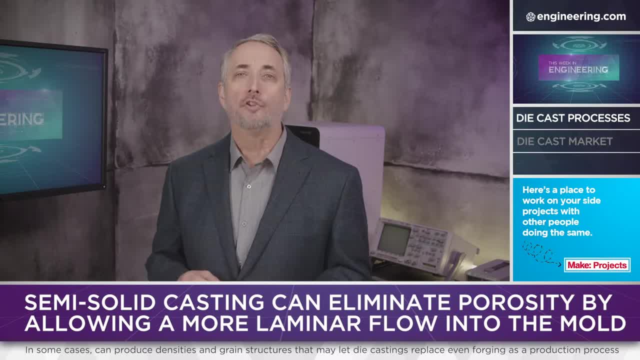 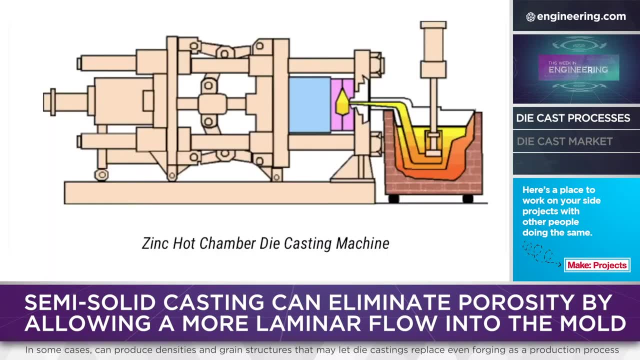 And in some cases it can produce densities and grain structures that may let die castings replace even forging. as a production process, In both semi-solid casting and die casting, metal is forced into a mold called a die, confusingly at high temperatures and pressures. 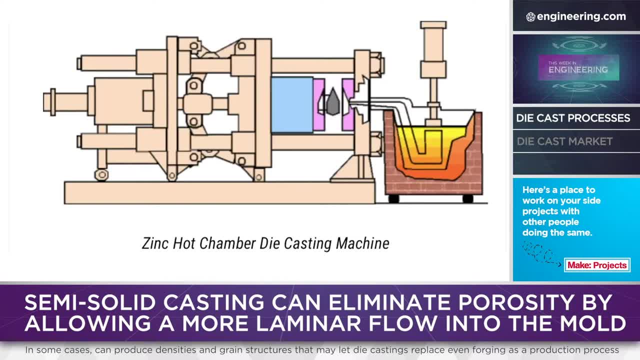 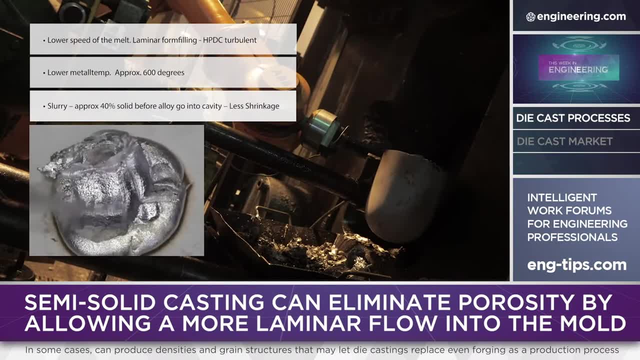 The key difference between die casting and semi-solid casting is that in die casting, the metal is in a fully liquid state, while in semi-solid casting the metal is between its solidus and liquid temperatures. You phase transition. people understand that This means that there's a mixture. 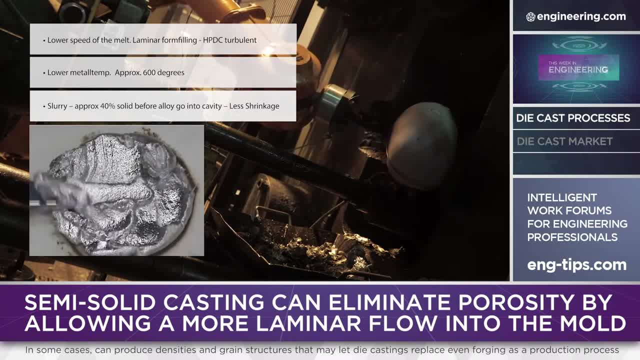 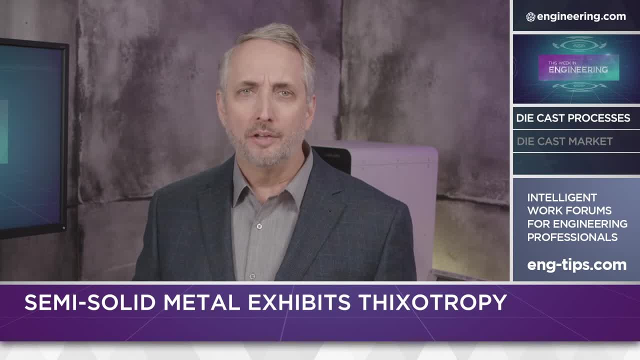 of solid phase globules surrounded by liquid metal. Now you can see this in a phase diagram. Now, in this state, the semi-solid metal exhibits something called thixotropy. This is a property where a fluid is relatively viscous when static, but it becomes less viscous when subjected to. 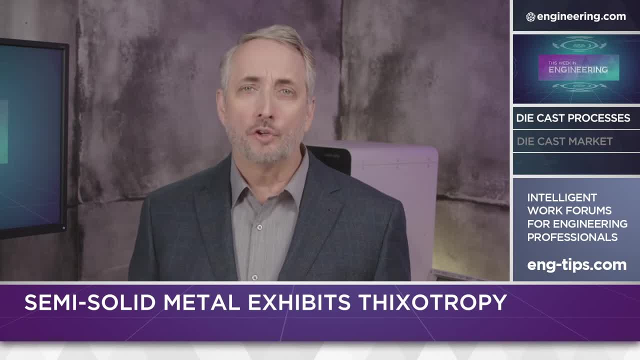 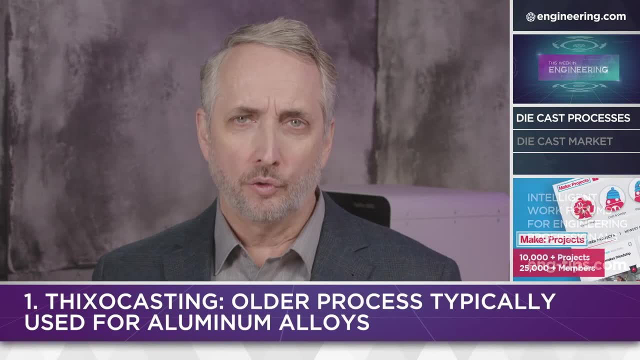 shear stress. The faster you shear the melt, the less force you need to apply, the more liquid the melt becomes. There are three distinct stages of this process. The first stage is called the distinct semi-solid casting processes, One fixo-casting. well, it's an older process. 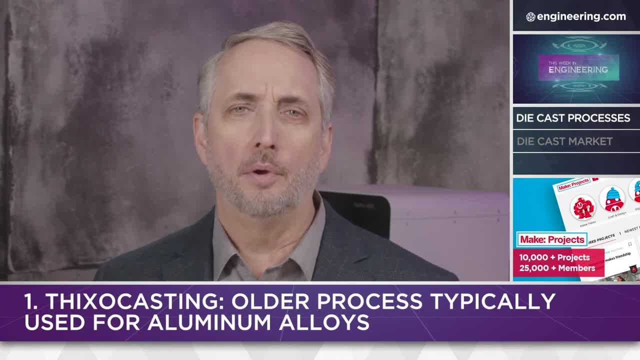 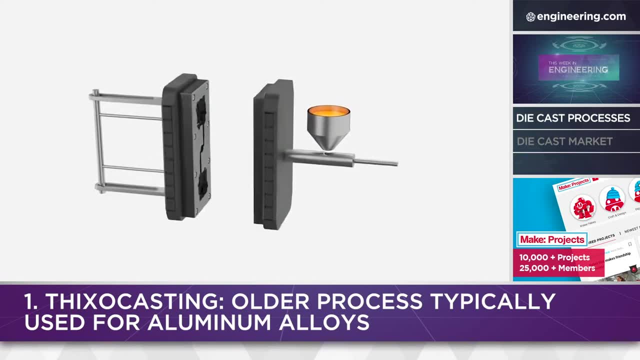 typically used for aluminum alloys. It requires a specially precast billet with a non-degeretic microstructure, adding significant cost to the process. This billet is then induction heated to form a semi-solid within a conventional die casting machine before being injected into a die. 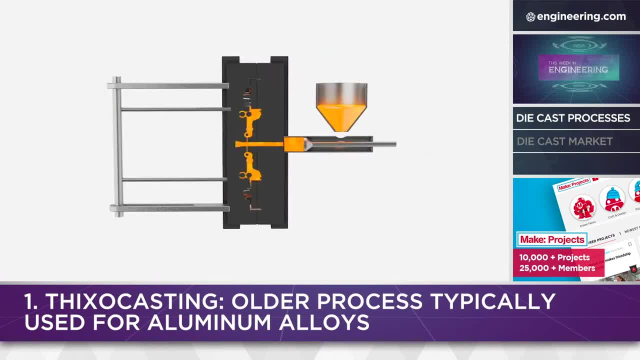 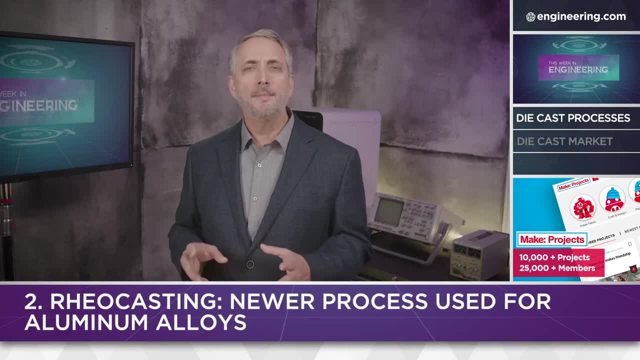 Now, this process makes it very difficult to reuse materials that must first be recast into that billet with the correct microstructure. Second, rheocasting is a newer process used for aluminum alloys. It uses the same casting machinery, furnace and handling automation as conventional die casting, but the difference is the addition of a. 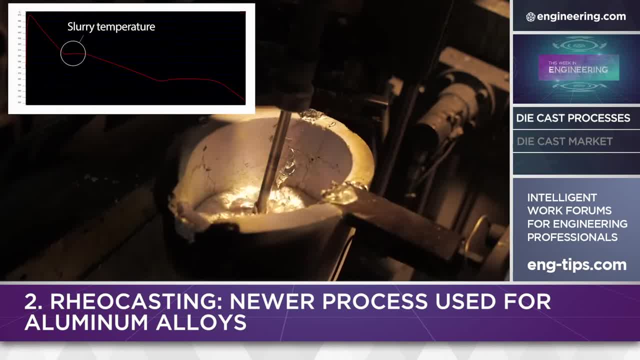 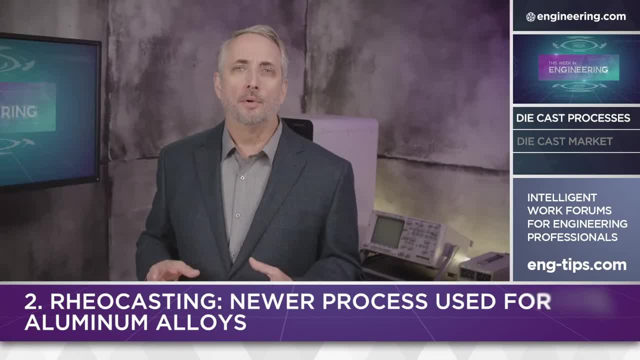 slurry maker, which is really a spindle that stirs the material in a crucible as it's being transferred from the furnace to the casting machine. The solid fraction is high, which is important for good results. And the third, fixo-molding. well, that's used for magnesium alloys primarily. It's 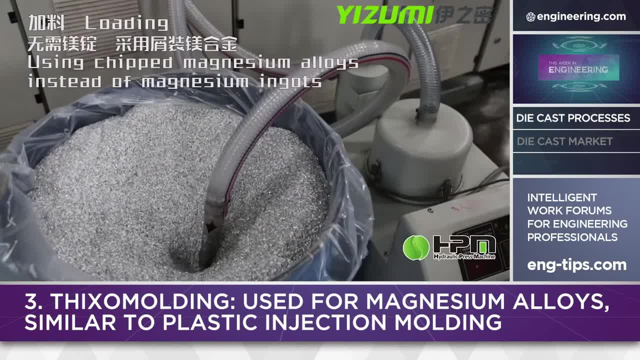 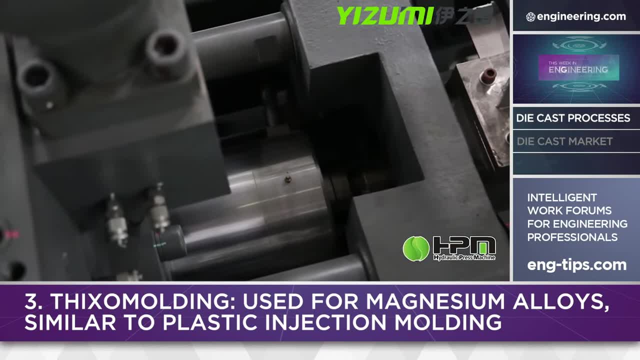 very similar to injection molding of plastics, with magnesium alloy chips fed into a barrel, where they're heated and metered using a screw conveyor. The action of the screw generates shear forces required for thixotropic thinning. There are many process and performance advantages to semi-solid. 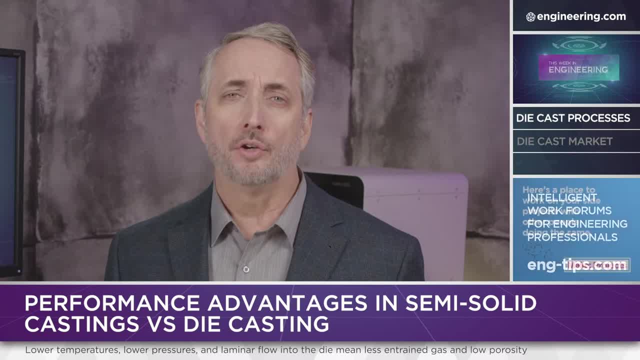 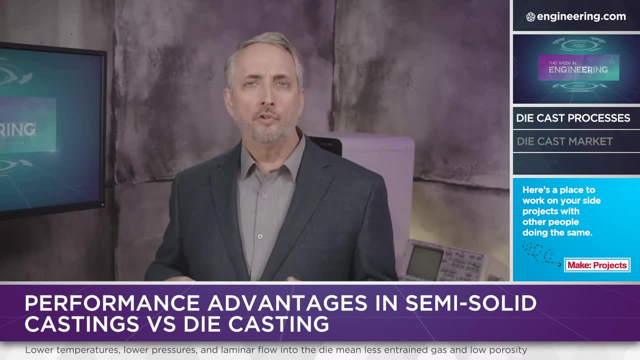 casting compared to conventional die casting: Lower temperatures, lower pressures and laminar flow into the die. well, that means less entrained gas and lower porosity. For many applications this is very important. Voids are potential stress risers and crack initiation sites. 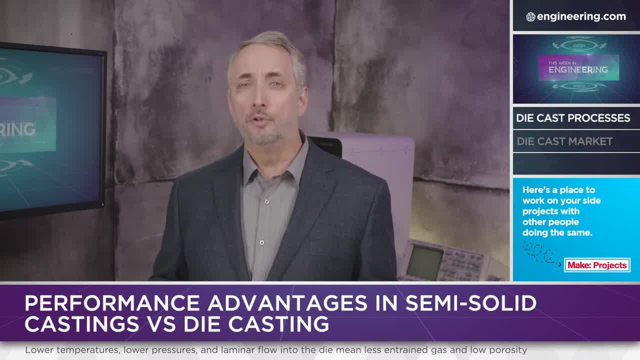 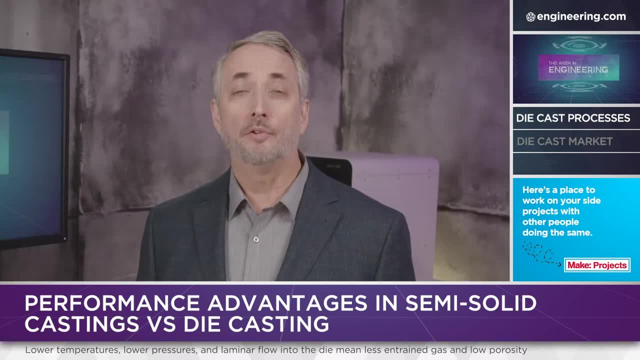 and a fully dense structure can allow the use of lower cost materials, reduce or eliminate post-processing or both. Another advantage is better fatigue life, along with that brittle fracture improvement, And it's possible to use alloys that are weldable. The lower temperature: 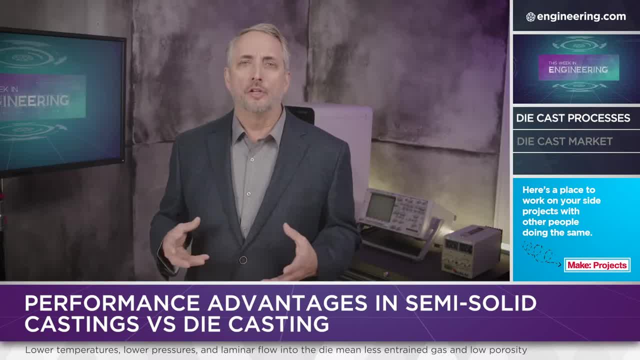 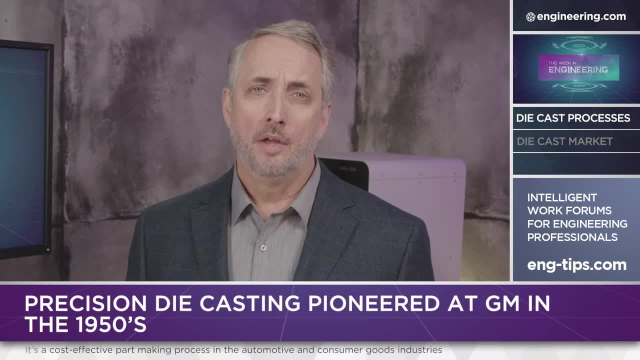 combined with a high proportion of solidity, means that there's less shrinkage. Now, this allows tighter tolerances to be maintained. Wall thicknesses can vary between less than a millimeter and over 20 millimeters. Now, precision die casting was pioneered at GM in the 1950s. 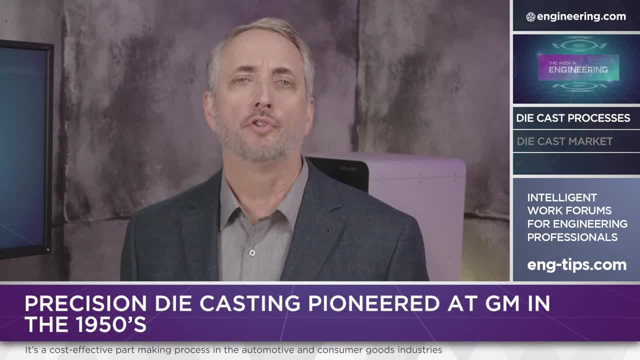 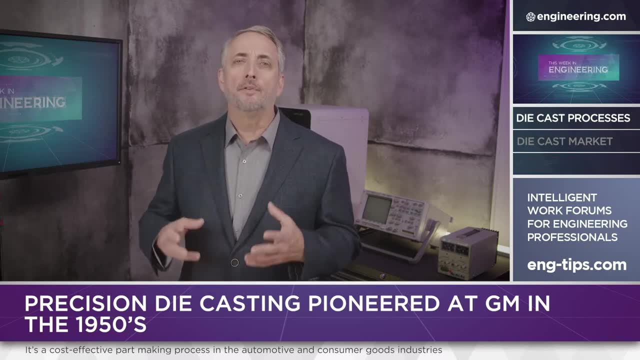 and it's been a cost-effective part-making process in the automotive and consumer goods industries ever, since Die casting for mass production uses relatively low melting point alloys of aluminum and zinc, and that lower temperature means tool wear is lower and one setup can operate for. hundreds of thousands of cycles. The automotive die casting market is expected to register a compound annual growth rate of more than 6.2%. Now, this is strong growth for a mature technology, especially with complex supply chain issues and the trend towards reshoring The auto industry. well, 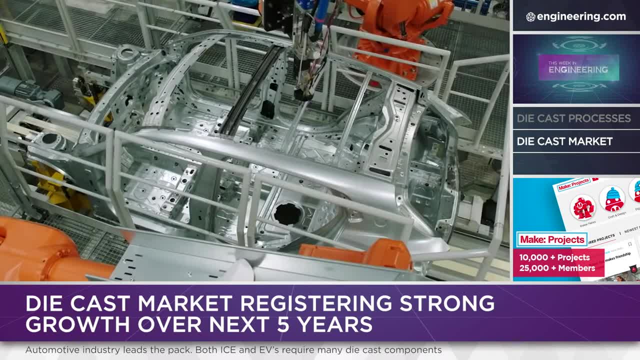 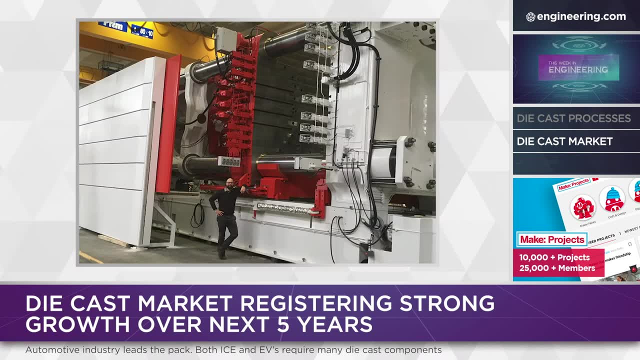 it's again the driver, with both internal combustion engine and electric vehicle technologies, carrying multiple components that can be cost-effectively die-cast in the chassis and the driveline. Now Tesla is attempting a gigantic die-cast subframe assembly as part of 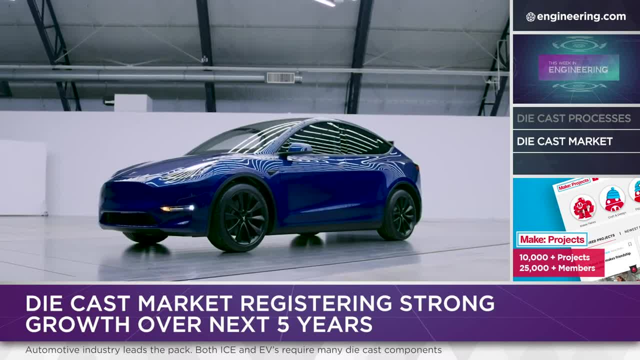 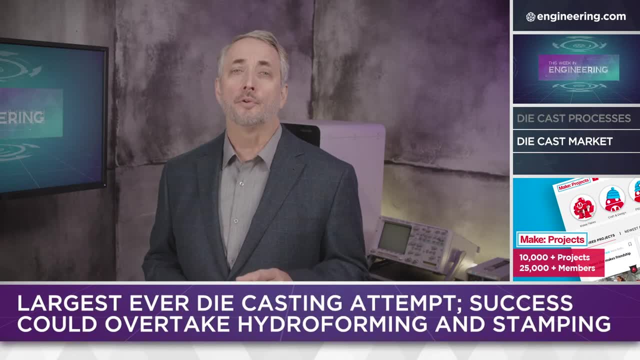 a new stressed battery pack structure for their new Model Y. This is to be built in the company's Berlin plan. This is the biggest ever attempted in this application. If it works it could make a lot more money than hydroforming or stamping in chassis design. Now, that's a big if, but this one.